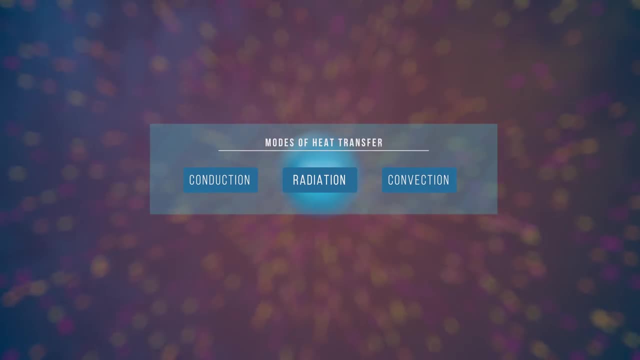 ways in which heat transfer can occur between different objects. Whether it's to design photovoltaic cells, heat exchangers or energy-efficient structures, engineers need to be able to model the effects of thermal radiation, And a good way to start is by taking a closer look at the electromagnetic waves themselves. 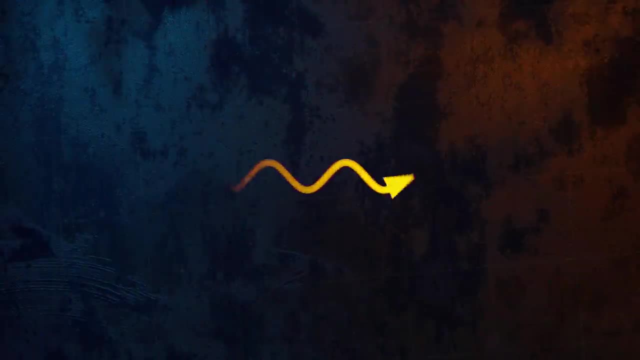 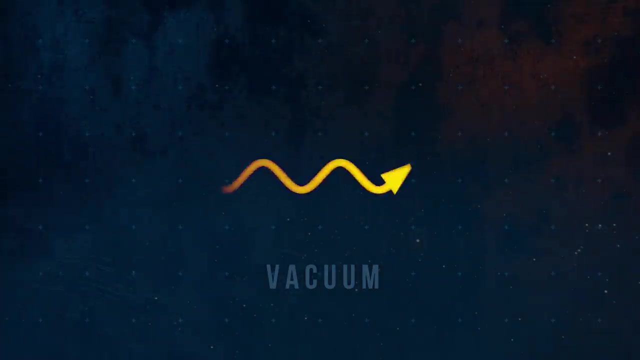 A first observation we can make is that these waves travel in a straight line from the emitter. They can also travel through a vacuum, which gives thermal radiation one of its most important functions. This means that each wave has its unique properties. unlike conduction and convection, it can occur in the absence of a medium. 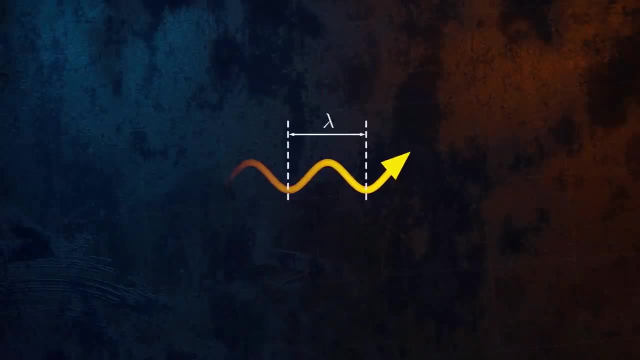 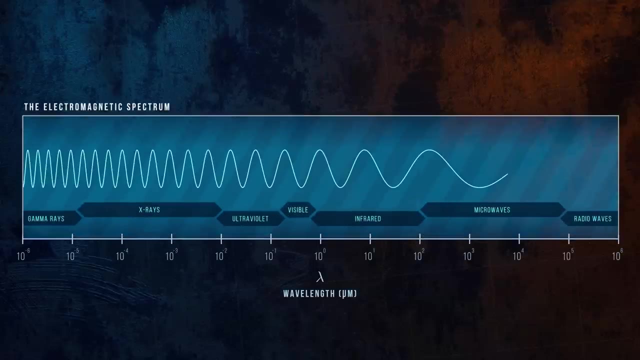 An electromagnetic wave is characterized by its wavelength. lambda Radio waves, for instance, are just electromagnetic waves with very long wavelengths are electromagnetic waves with short wavelengths. Visible light has a wavelength between around 0.4 and 0.7 microns. 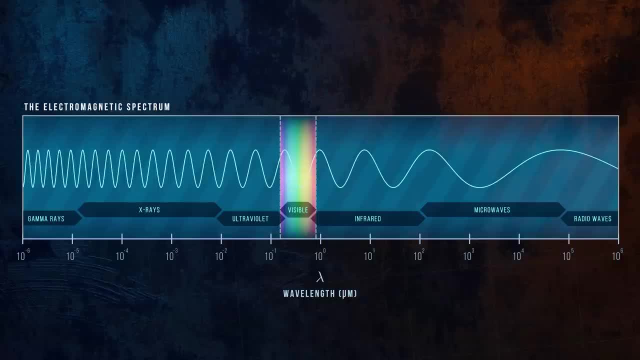 The thermal radiation emitted by an object due to its temperature has a wavelength between 0.1 and 100 microns. It overlaps with the UV, visible and infrared parts of the spectrum: The total energy radiated by a body each second. 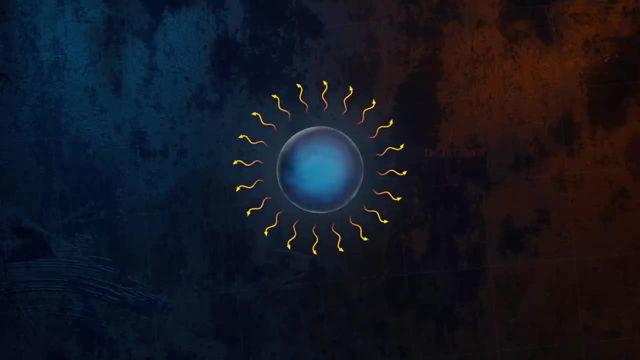 per unit area is called the emissive power E. It has units of watts per square meter. To study thermal radiation, it's useful to define a perfect emitter that emits the maximum possible amount of thermal radiation at a given temperature. This theoretical definition of thermal radiation is based on the theory that it is possible to 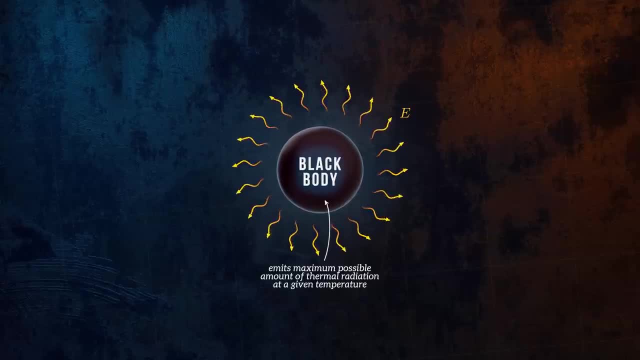 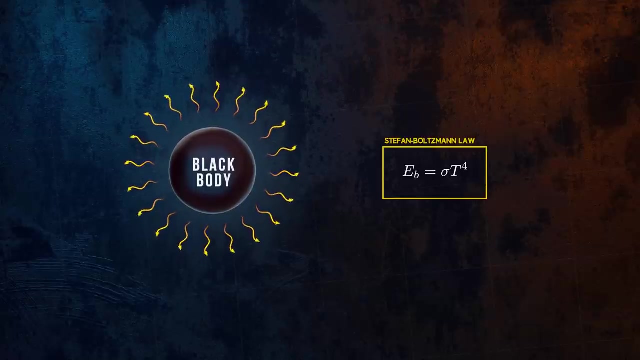 calculate the emissive power of a black body using a surprisingly simple law called the Stefan-Boltzmann law. T is the absolute temperature in Kelvin and sigma is a constant called the Stefan-Boltzmann constant Multiplying the emissive power. 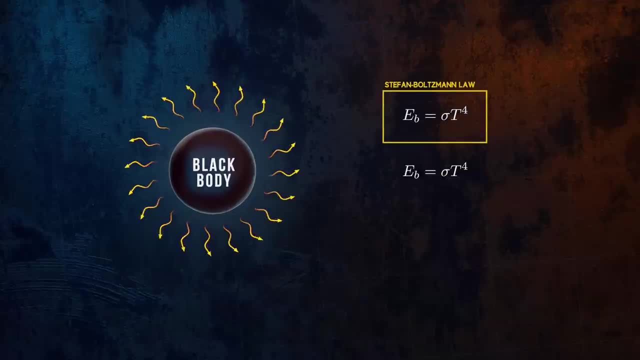 by the surface area of the body gives us the heat transfer rate. A spherical black body with a radius of 30 centimeters at 300 Kelvin, for example, will emit heat at a rate of 520 watts or 520 joules per second. 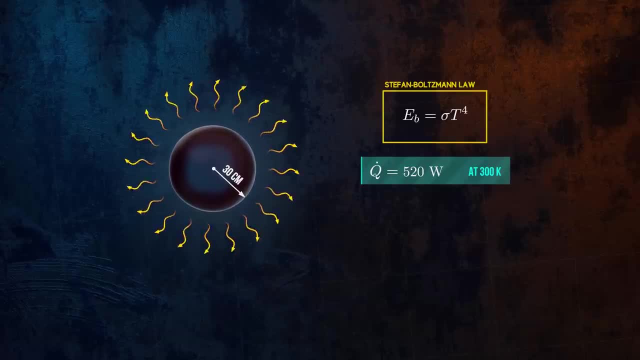 Temperature in the Stefan-Boltzmann law is raised to the fourth power. This means that bodies at high temperatures emit far more energy by radiation than those at lower temperatures. Increasing the temperature of the sphere to 600 Kelvin will cause it to radiate 16 times more. 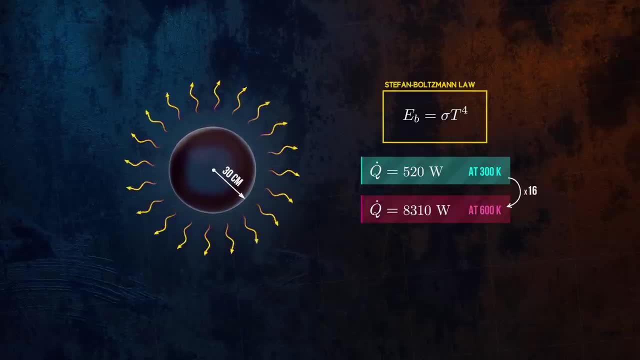 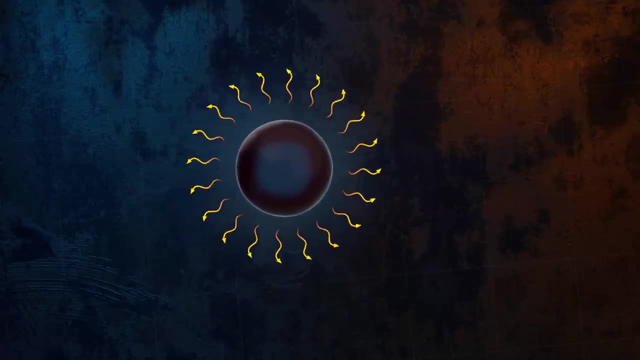 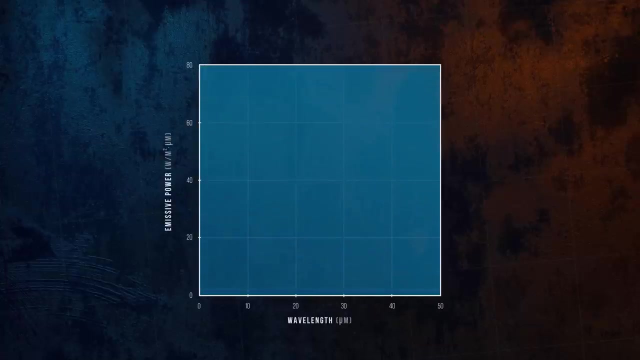 energy each second. The electromagnetic waves emitted due to thermal radiation don't all have the same wavelengths. For the black body with a temperature of 300 Kelvin, the radiated energy is in the form of electromagnetic waves with wavelengths mainly between 10 and 40 Kelvin. 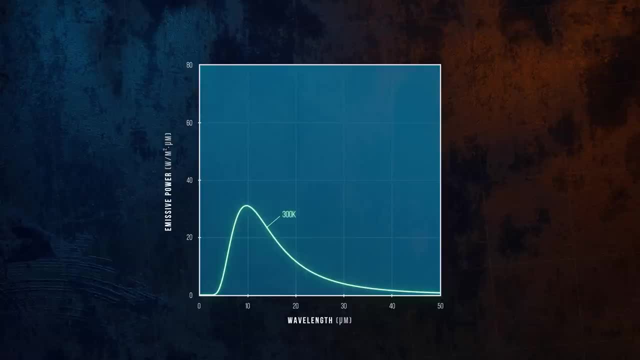 and 50 microns. The total emissive power which we saw earlier can be calculated by the Stefan Boltzmann law. can be obtained from this graph by summing up all of the contributions from each wavelength, which is just integrating, to obtain the area under the curve. 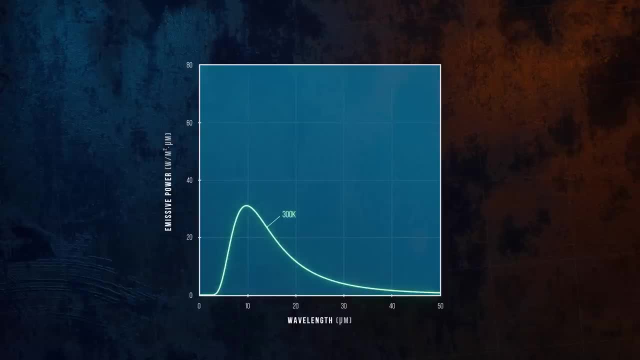 At 300 Kelvin, none of the emitted energy is in the visible part of the spectrum. As the temperature of the blackbody increases, the total emissive power increases very quickly, so we'll need to switch to a log scale graph to be able to compare distributions for different. 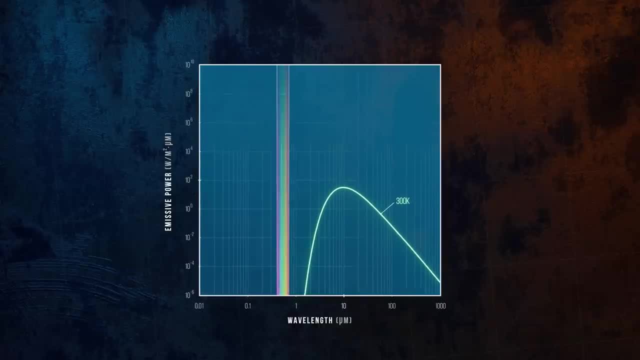 temperatures. As temperature increases, the distribution shifts to the left, meaning that the emissive power is made up of shorter and shorter wavelengths. Starting at around 700 Kelvin, we reach the visible part of the spectrum, which is why objects begin to glow when they reach high enough temperatures. 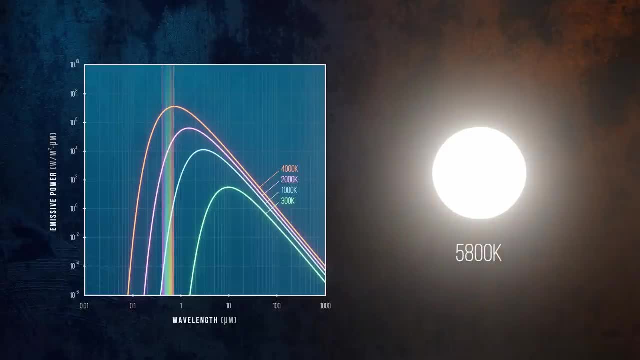 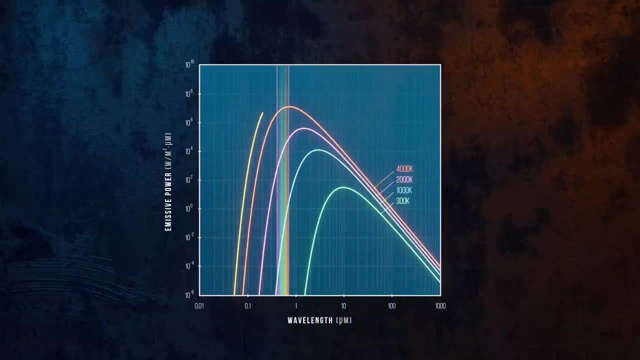 The surface of the sun can be modeled as a blackbody with a temperature of 5,800 Kelvin, and the wavelengths that emit the most radiation fall within the visible range of the spectrum, although it emits a lot of energy in the UV and infrared wavelengths too. 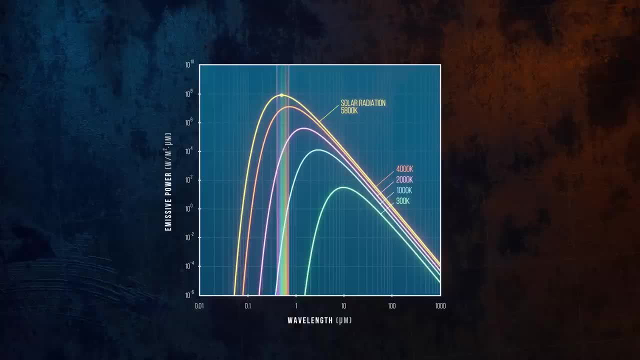 The wavelength at which most of the power is emitted is often of interest. it varies with temperature and is given by a relation called Wien's Displacement Law. Wien's Law is often applied in astronomy If we measure the light emitted by a distant star. 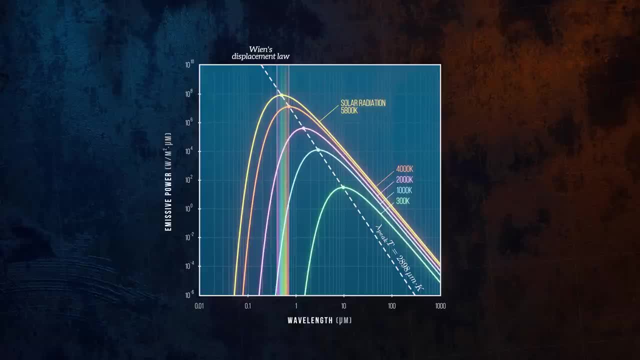 for example, we can determine the wavelength at which the maximum power is emitted, and so, by assuming the star behaves as a blackbody, we can determine its surface temperature. The Distribution Source- Distributions we've looked at so far only apply to blackbodies. 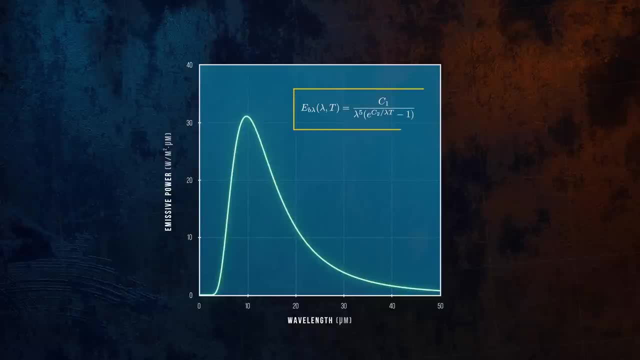 They're defined by Planck's Law, But it's important to remember that a blackbody is an idealization. Some real bodies do behave similarly to blackbodies, but for most the spectral emissive power profile will look something like this: 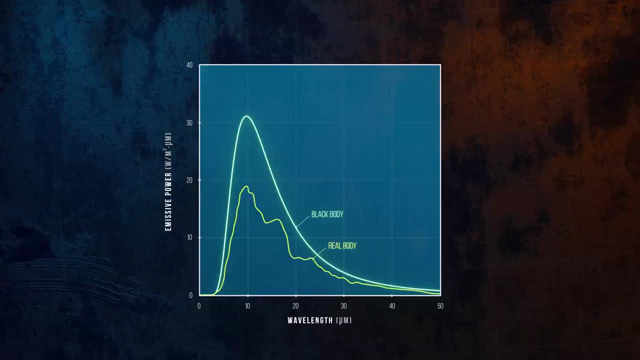 Since the blackbody is an idealization of the perfect emitter. since the blackbody is an idealization of the perfect emitter, the emissive power of the real body is less than that of the blackbody. We can still use the Stefan-Boltzmann Law to calculate the emissive power of a real body. 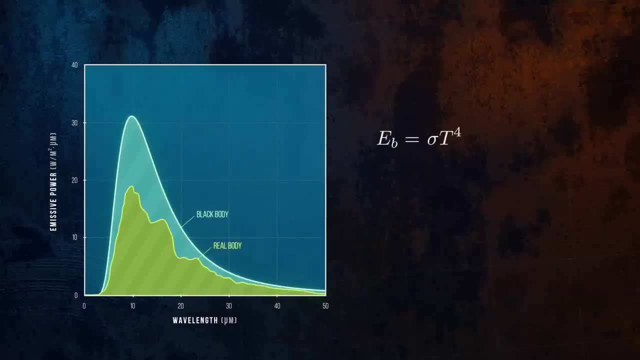 We just need to include an additional term, the emissivity epsilon, That defines how much the real body emits relative to a blackbody. It's defined more formally as the emissive power of the real body divided by the emissive power of a blackbody at the same time. 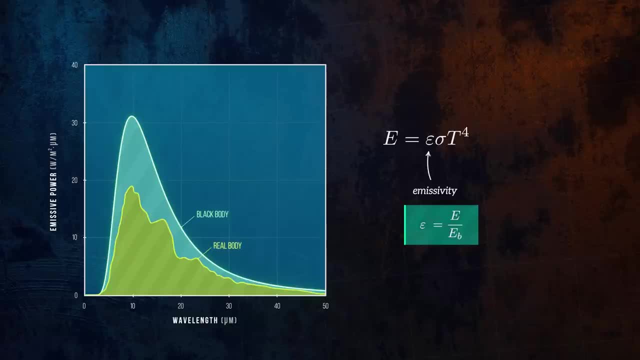 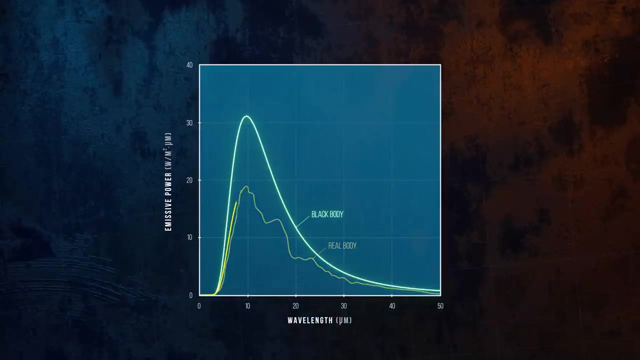 Emitivity values, which tend to vary with temperature and wavelength, can be found in reference texts or can be determined experimentally. A body is said to be a gray body if the emissivity is constant for all wavelengths. This is a simplification that makes it easier to analyze real bodies. 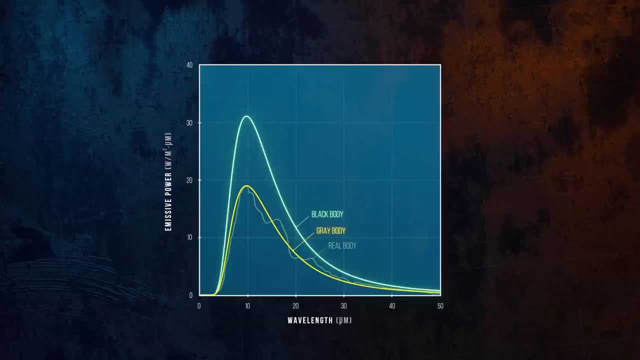 For an opaque body, thermal radiation is very much governed by the emissivity. For an opaque body, thermal radiation is very much governed by the emissivity the properties of its surface. so coating type and surface roughness significantly affect emissivity. In fact, surface emissivity is often an important consideration when making design decisions. 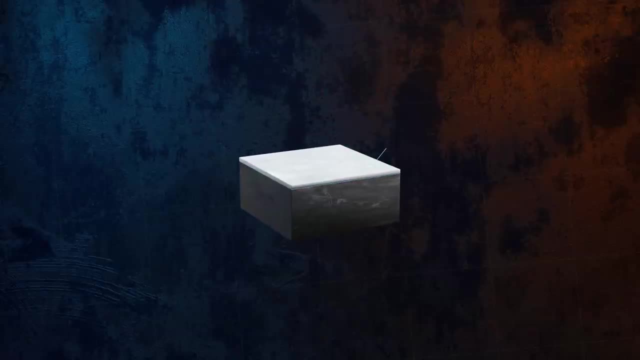 A metallic coating with a polished surface finish will have very low emissivity and so might be a good choice for the surfaces of a heat tank, as it will reduce the amount of heat radiated to the environment, but it probably won't be a good choice for an electronics. 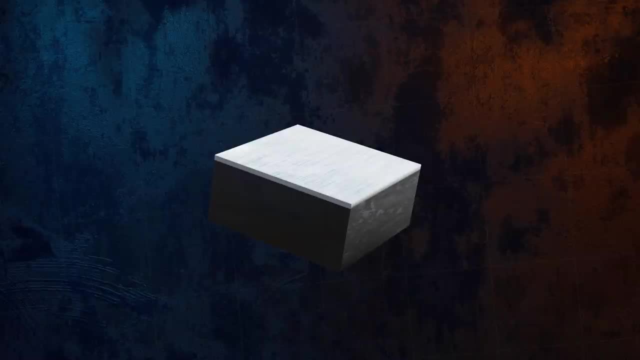 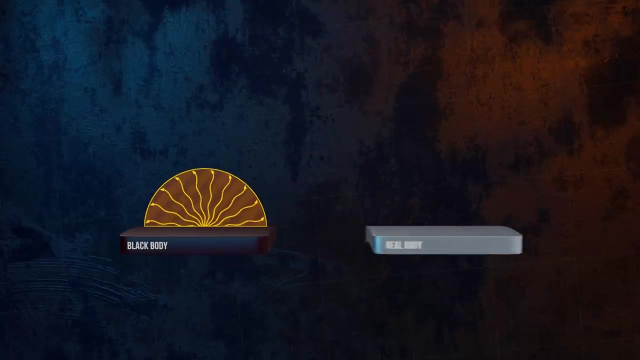 enclosure that needs to be able to radiate heat effectively. Another idealization assigned to a blackbody is that it's a diffuse emitter, meaning that it emits radiation evenly in all directions, But real surfaces tend to emit radiation unevenly, So what's the difference? 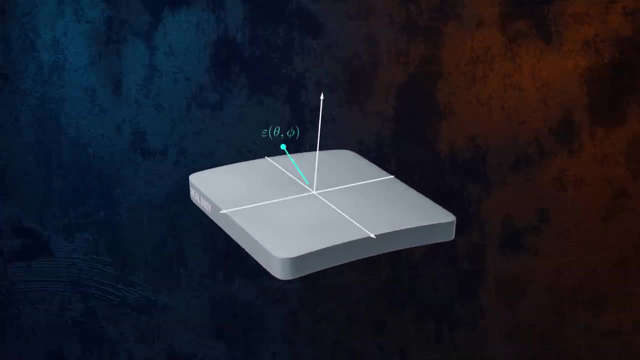 The emissivity is then a function of the angles theta and phi, although it varies mainly with the angle theta. Capturing this directional dependence in a heat transfer analysis can get quite complex, but fortunately it's often reasonable to assume that objects act as diffuse emitters. 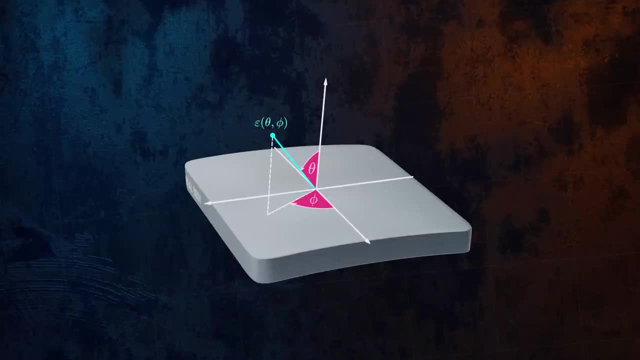 and to use either an average emissivity or the emissivity in the direction normal to the surface. Of course, when studying radiation, we don't only care about how much power an object emits. we mainly care about the interactions between different bodies, and emission is only one. 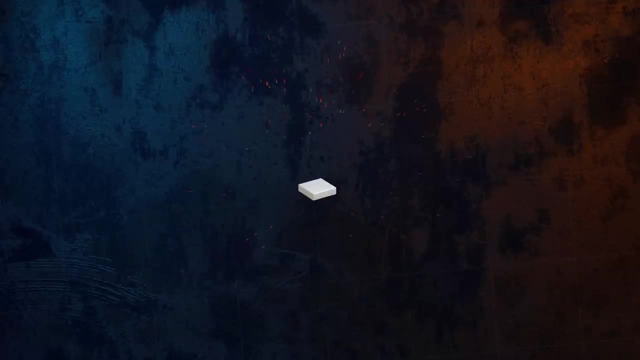 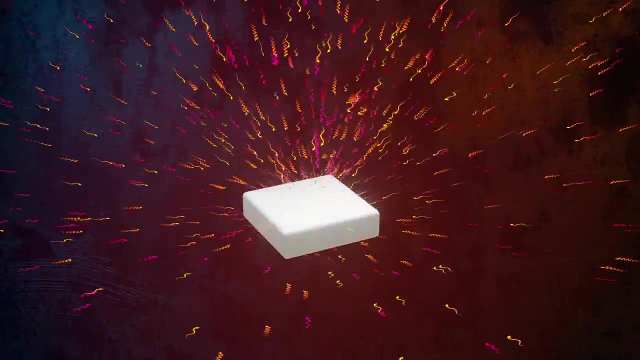 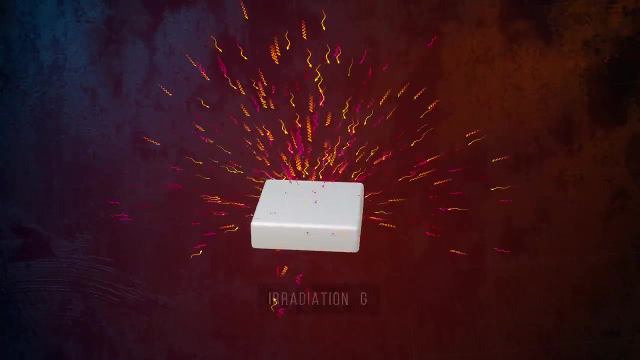 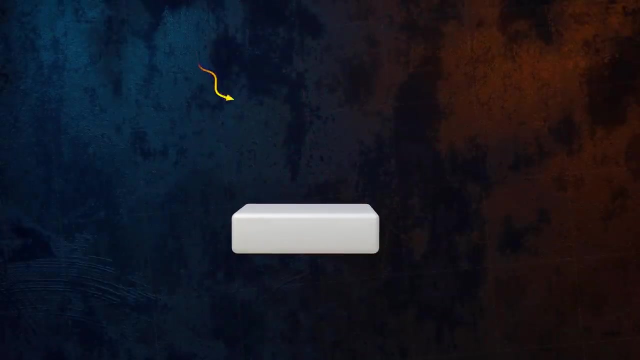 part of that. The total amount of thermal radiation that reaches a body and per unit area, regardless of where it originates from, is called irradiation, and it's denoted using the letter G. That's it. When radiation reaches the surface of an object, three things can happen. 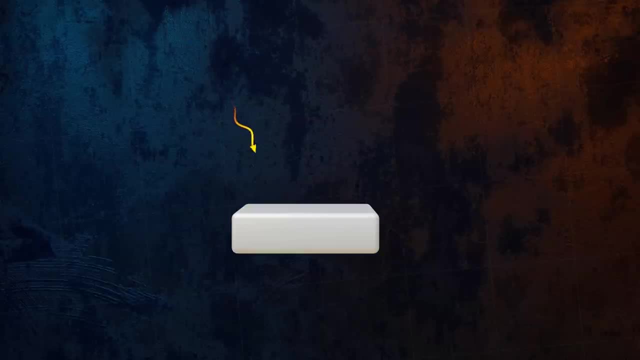 The waves can be absorbed, which increases the temperature of the body. They can be reflected or, in the case of a body that isn't completely opaque, they can also be transmitted through it. The proportion of the total irradiation reaching a surface that is absorbed, reflected or 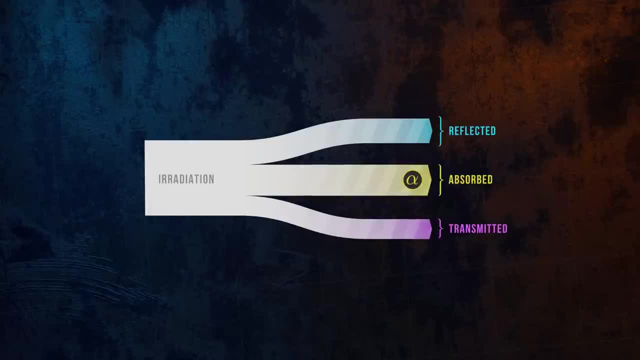 transmitted is described by the absorptivity alpha, the reflectivity rho and the transmissivity tau. Values for these parameters will differ depending on the surface, material and finish and, like the emissivity epsilon, they can be found in reference material or be determined experimentally. 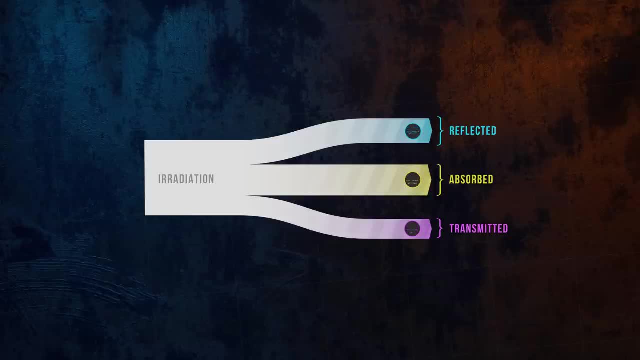 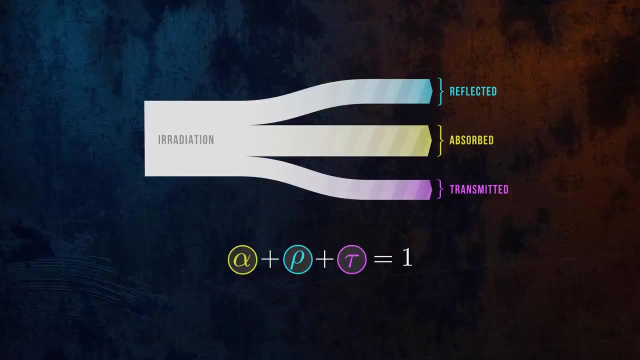 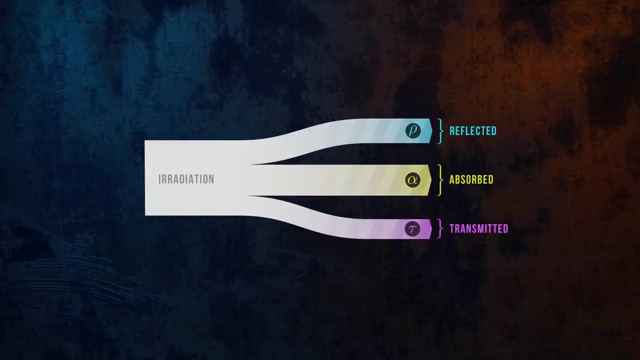 Since all incident, energy is either absorbed, reflected or transmitted, these three terms must sum up to one. As well as being a perfect emitter, a black body also absorbs 100% of the radiation incident upon it, So it has an absorptivity of 1, and the reflectivity and transmissivity are 0. 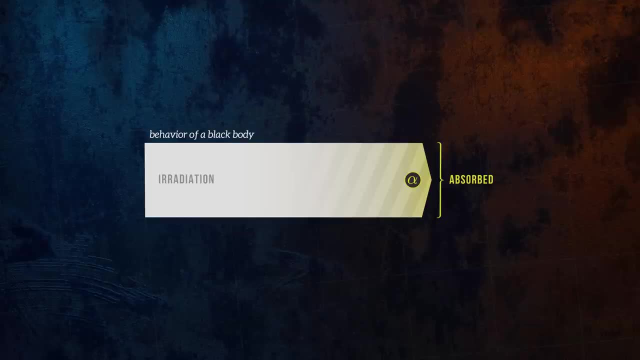 This is where it gets its name: It absorbs all of the light that hits it and so appears to be black, as long as it's not emitting radiation in the visible part of the spectrum, Like for emissivity- Emissivity- Emissivity. 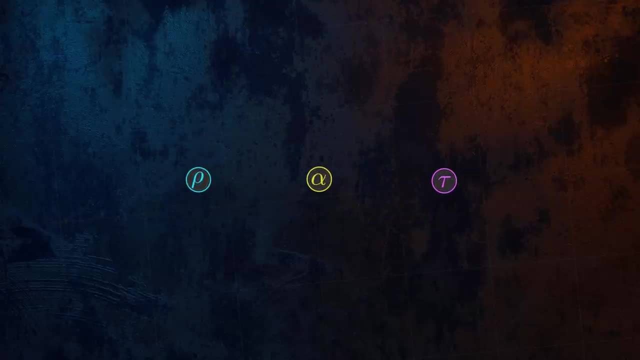 Relativity, reflectivity and transmissivity are typically functions of wavelength and direction. We're getting closer to being able to model radiative heat transfer between different objects, but there's one last thing we're missing. The way radiation is exchanged between surfaces depends on how the surfaces are positioned. 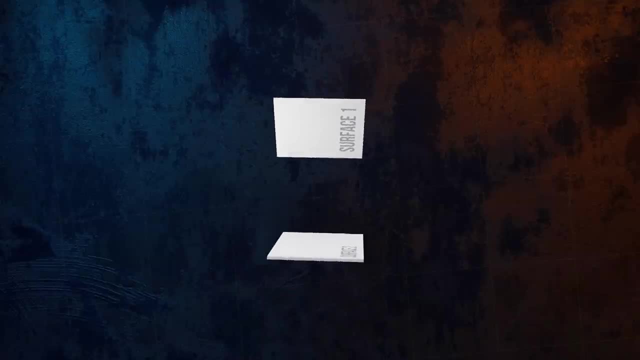 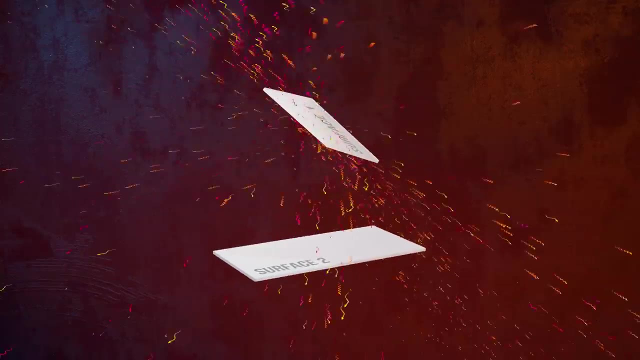 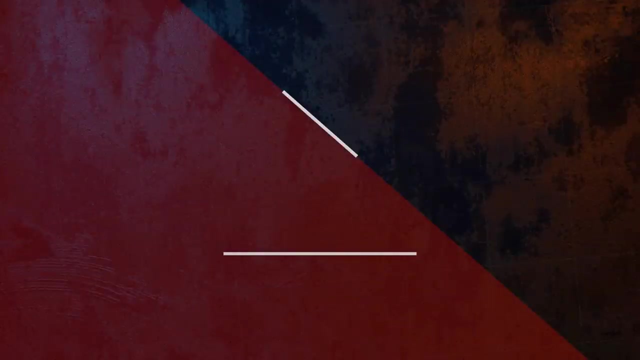 relative to one another. Assuming that surface 1 is a diffuse emitter and so emits thermal radiation evenly in all directions, all of the radiation it emits will be in this area shown in orange, But only a fixed portion of this radiation will ever reach surface 2.. 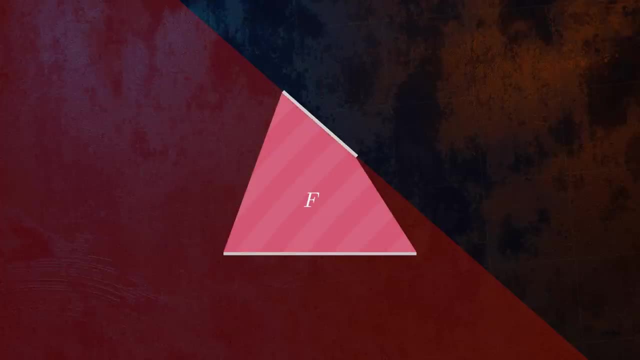 We can define a parameter F that describes the fraction of energy radiated from surface 1 that reaches surface 2.. This is called a shape factor or view factor. It's a purely geometric parameter that depends on the shape of the surfaces and how. 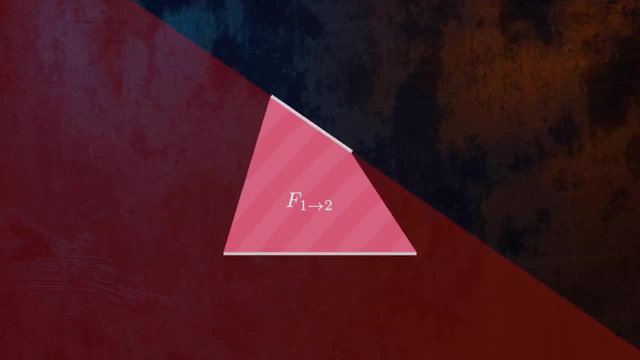 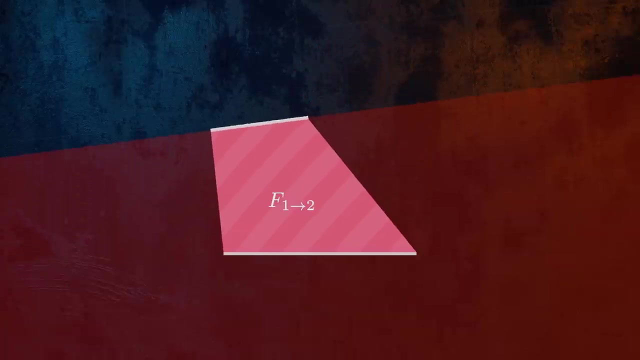 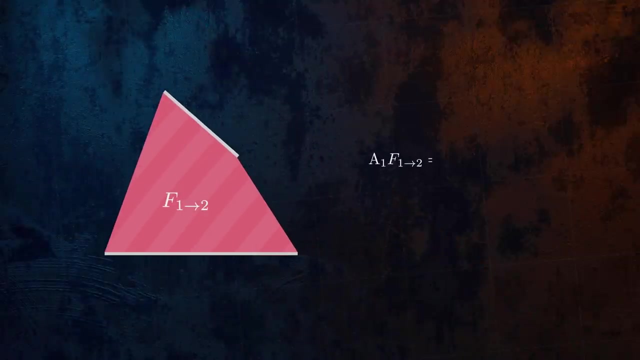 they are oriented relative to one another. A relation called the reciprocity rule gives us an equation relating the view factors and areas for both surfaces. This means that if we know the view factor in one direction, we can easily determine the shape of the surfaces. 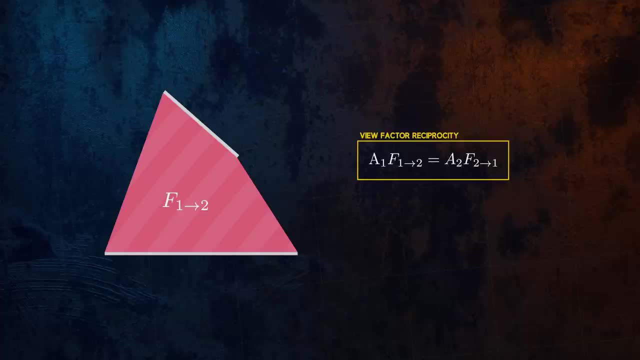 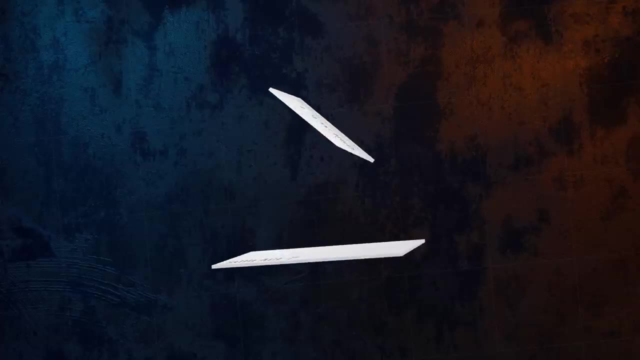 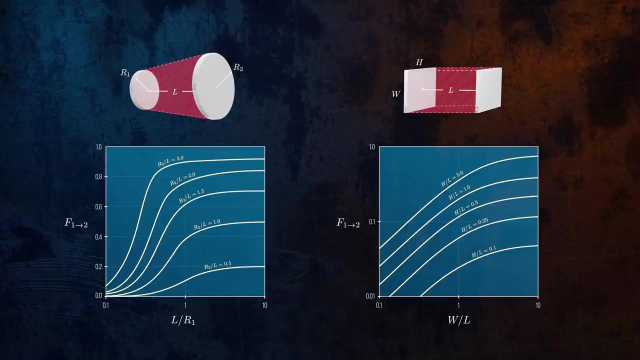 We can easily calculate it in the reverse direction. View factors can only really be calculated analytically for very basic cases. Charts and tables are provided in reference texts for many simple configurations, But specialist software needs to be used for more complex scenarios. Once we have the view factor, we can calculate the heat exchange between the two surfaces. 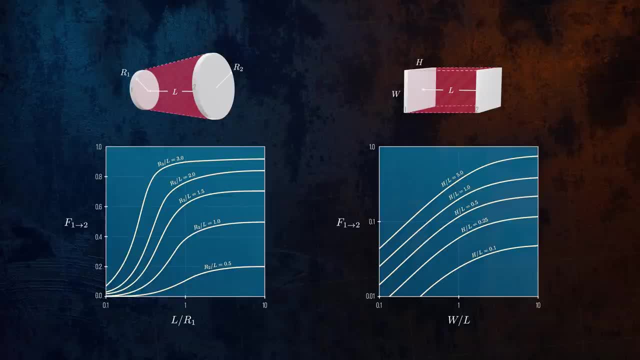 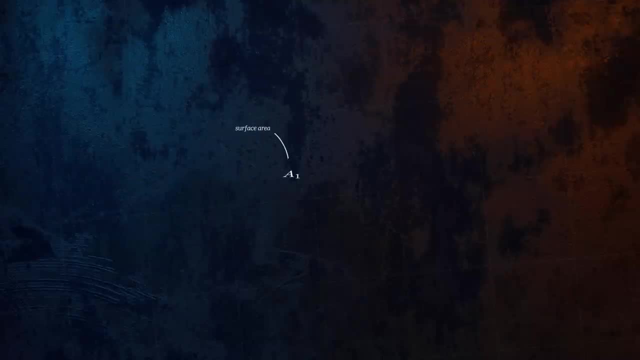 Survey result. If we assume both surfaces behave as black bodies, the total radiation that leaves surface one and reaches surface two is the product of the area of surface one, the black body emissive power of surface one and the view factor from surface one to surface two. 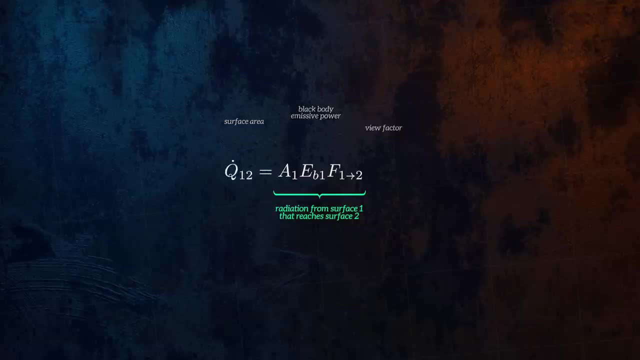 We can then calculate the net heat transfer between the two surfaces by subtracting the radiation that leaves surface two and reaches surface one. futher details 苦. The emissive power Eb is defined by the Stefan-Boltzmann law and applying the reciprocity relation. 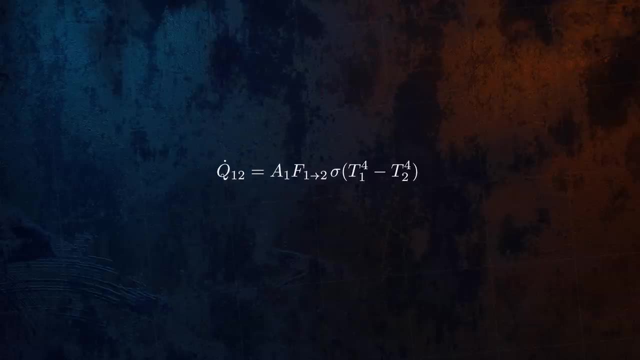 gives us this simple equation for the net rate of heat transfer between both surfaces. Things get a bit more complicated if we assume the surfaces behave as grey bodies, because it means we have to consider reflection. To do this, we can replace the black body emissive power, Eb, in the heat transfer equation. 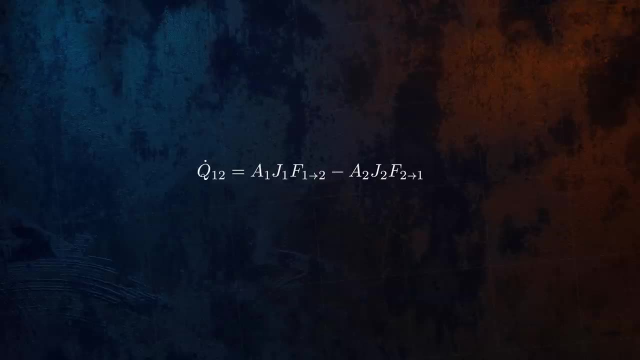 with a new parameter, the radiosity J. Radiosity is the total radiation that leaves a surface and is the sum of the emitted and the reflected portions. Analyzing radiation can get complicated very quickly, but we've covered the key concepts that can be used as a starting point for dealing with more complex scenarios. 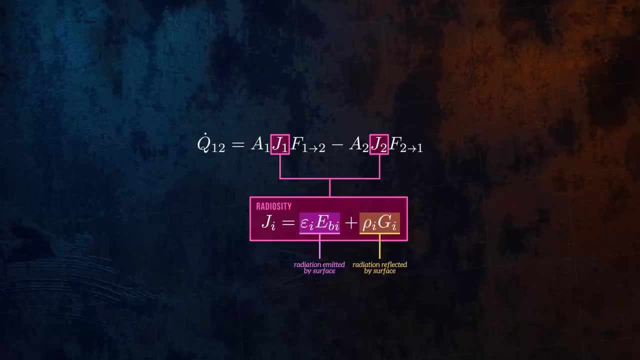 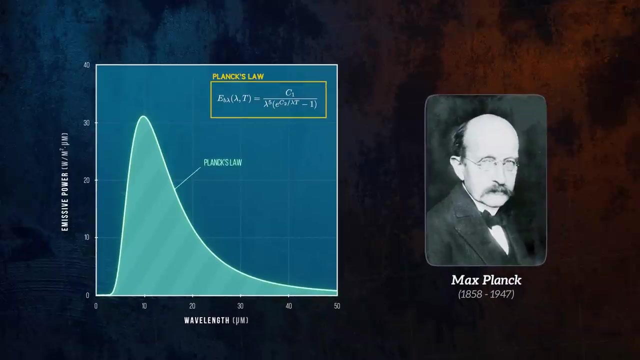 Thanks for watching. So far we've described radiation as electromagnetic waves, but the reality is much less straightforward. Planck's law that defines the distribution of the emissive power of a black body was derived by Max Planck at the beginning of the 20th century. 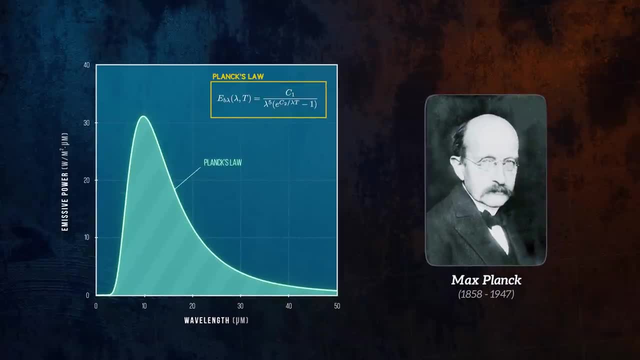 Until then, classical physics predicted distributions that looked vastly different to experimental measurements at short wavelengths. This unexplained discrepancy between the models is the result of a series of experiments to determine how much radiation is emitted by a black body, and how much radiation is emitted. 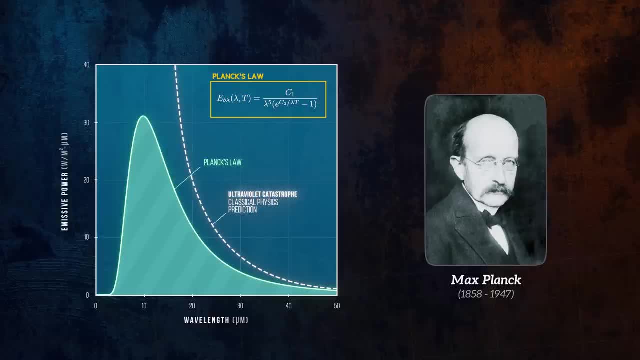 by a black body. The difference between the models and the data was called the ultraviolet catastrophe. Planck solved this by considering that radiation might not actually be emitted continuously, as had been assumed by the classical models, but instead that it's emitted in discrete. 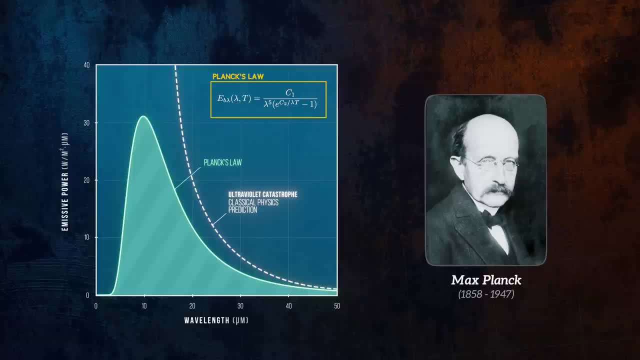 packets of energy that we now call photons. This theory led to a much closer match with the experimental data, and the revolutionary discovery that light is quantized opened the doors to the entire field of quantum mechanics. If you're interested in learning more about Max Planck and the early days of quantum, 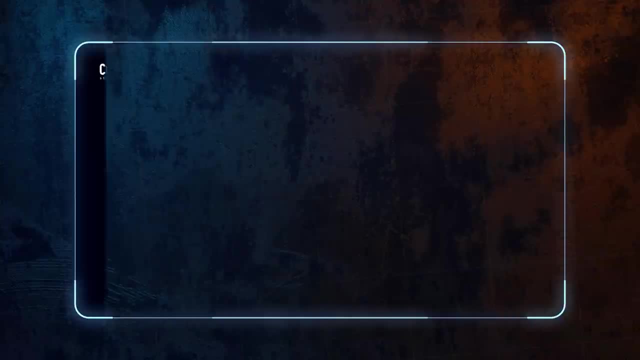 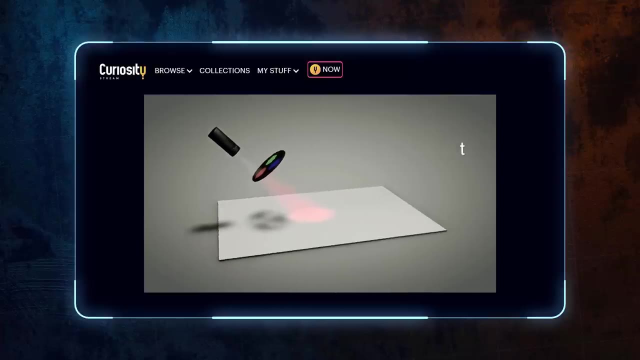 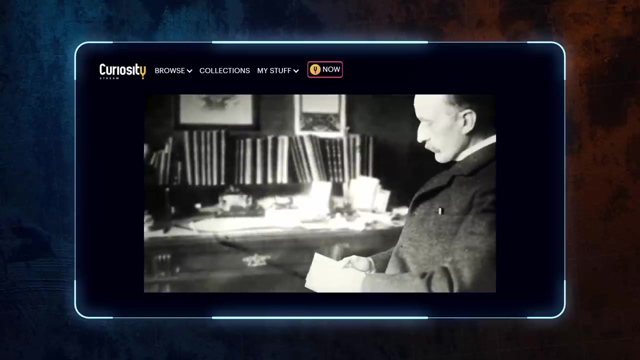 mechanics. I highly recommend you check out the documentary series Exploring Quantum History from CuriosityStream, who have kindly sponsored this video Hosted by physicist Brian Greene. it covers the early work done by Planck, but also the key contributions from Albert Einstein, Werner Heisenberg and Niels Bohr, and it explores 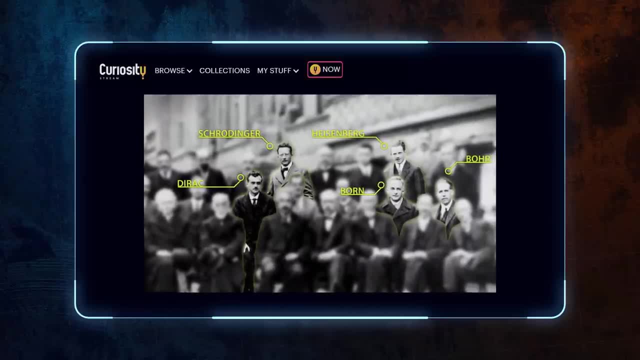 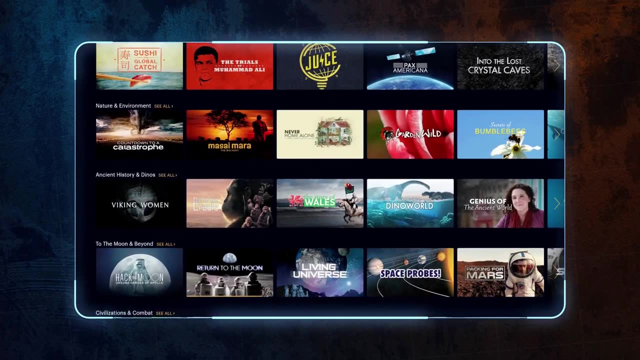 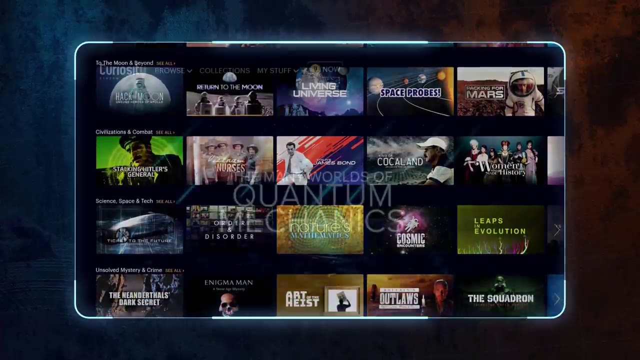 how quantum mechanics might shape the future. CuriosityStreamcom. Thanks for watching. CuriosityStream is an amazing documentary streaming service that has a huge catalog containing thousands of titles. There are several other documentaries about quantum mechanics on there, including a great one about the many worlds interpretation of quantum mechanics, but also countless others. 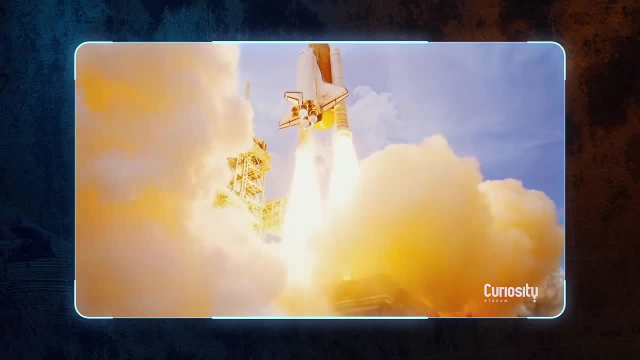 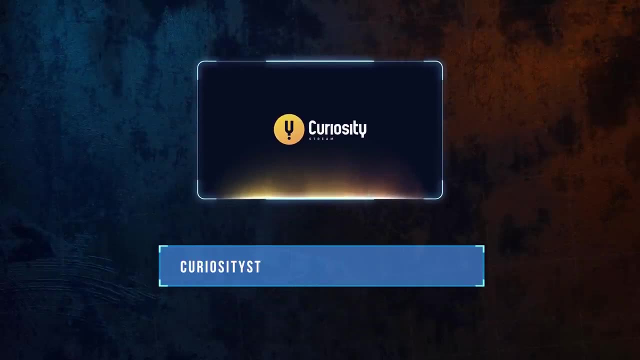 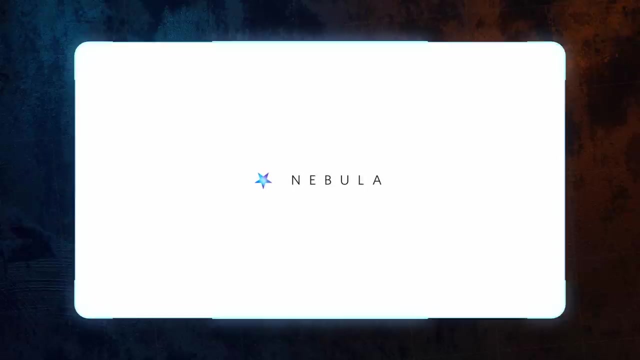 covering the natural world, science, technology and more. If you sign up using this link, you'll get a 26% discount on the annual plan, but there's more. You'll also get a full subscription to Nebula, which, I'm sure you know by now, is the streaming. 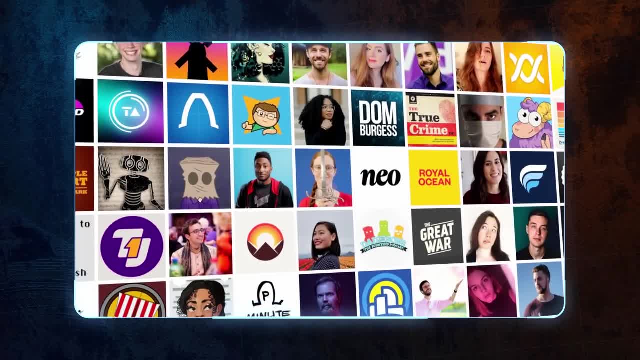 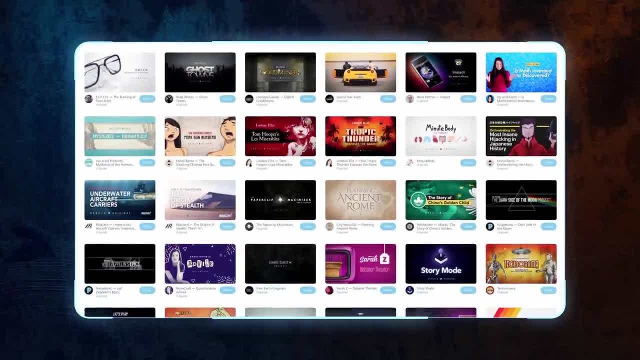 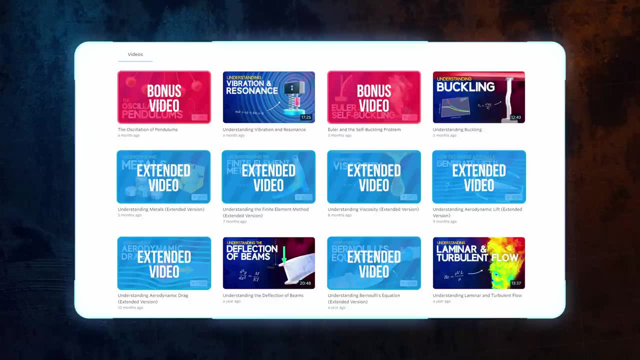 service a group of independent educational creators, including myself, have been building. Nebula is a place where we can experiment with new ideas and upload bonus content, all without worrying about the YouTube algorithm. In fact, I've just uploaded a full-length video exclusively to Nebula, covering dimensional 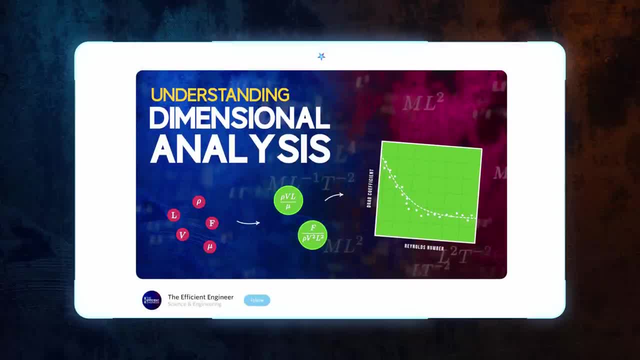 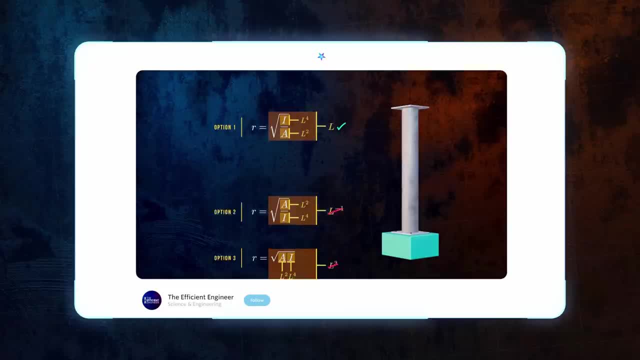 analysis An incredibly powerful analytical technique. I hope you enjoy it. It's a brilliant analytical technique that engineers can use to sense-check equations, identify the important parameters in a problem and even derive completely new relations based on experimental data. It's particularly important for the study of fluid mechanics and heat transfer, where